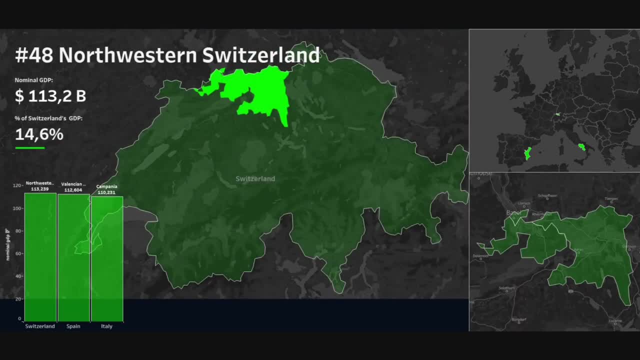 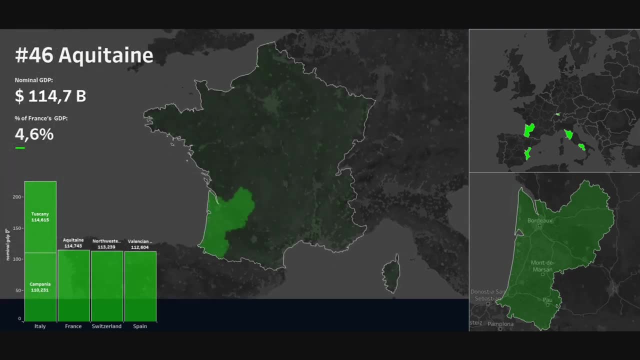 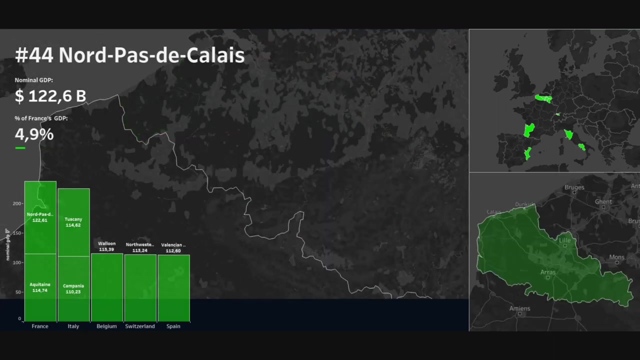 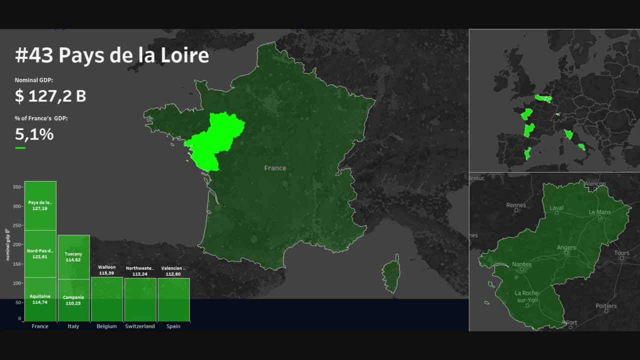 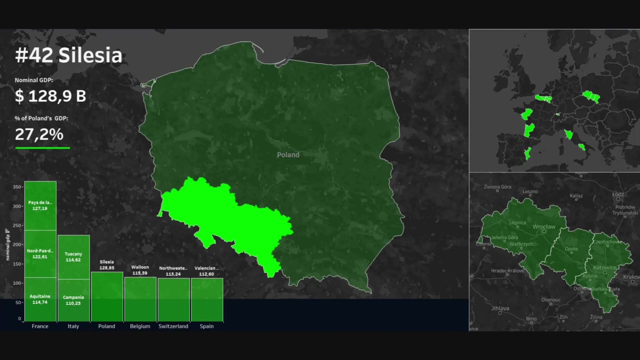 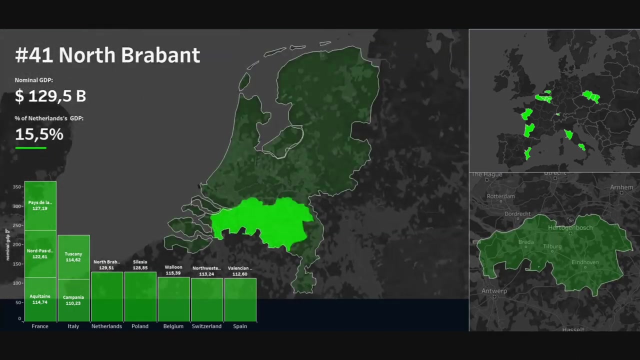 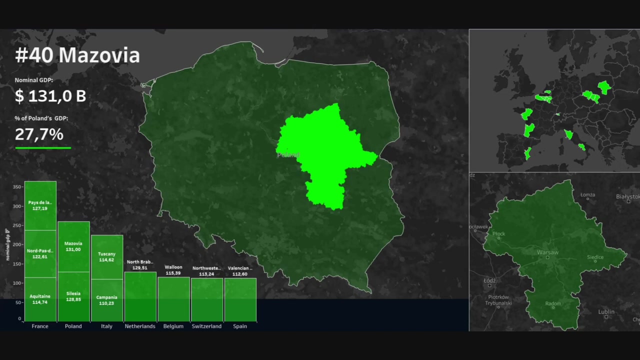 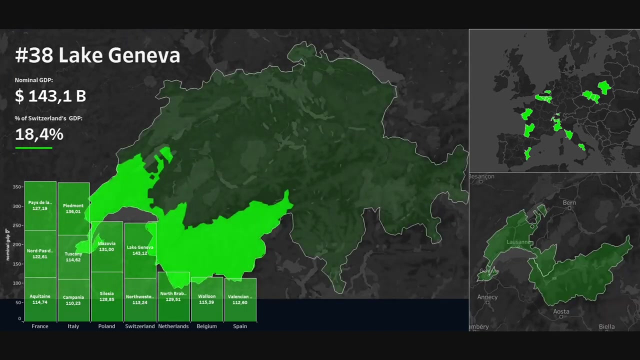 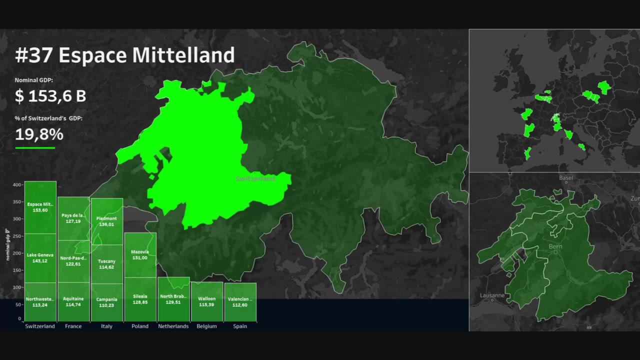 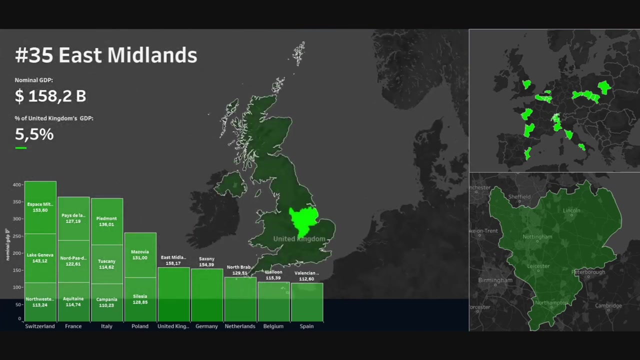 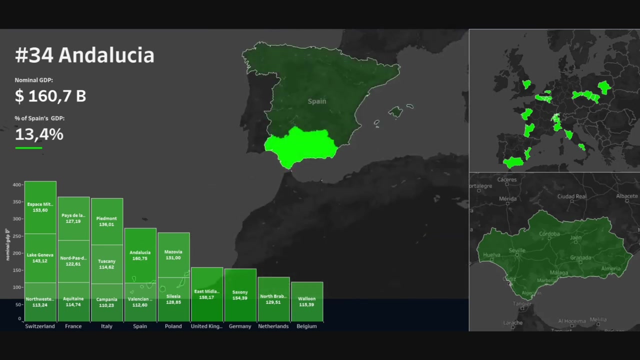 We are moving forward at an accelerated pace. Saliza is a real powerhouse of Polish industry. It is home to many factories and mining mines. However, the region is now developing in the direction of providing services. attacks were made in modern Greece earlier this year as the Greek messengerивал. 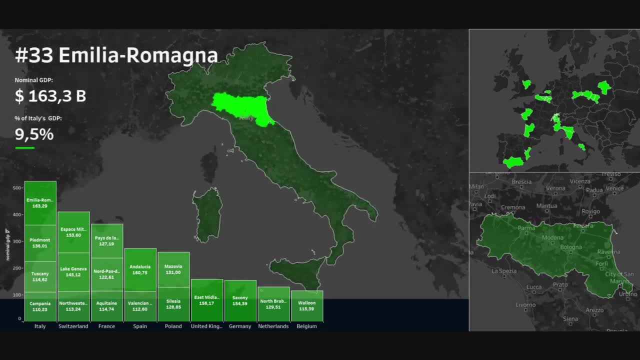 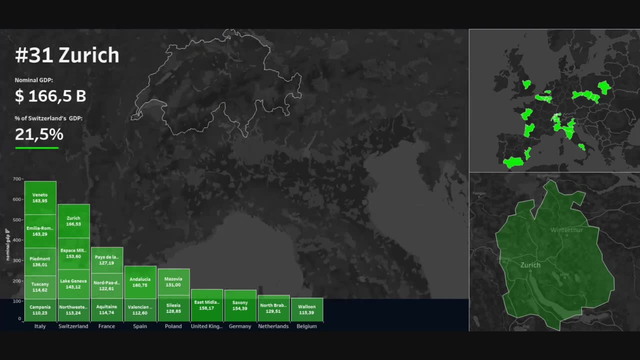 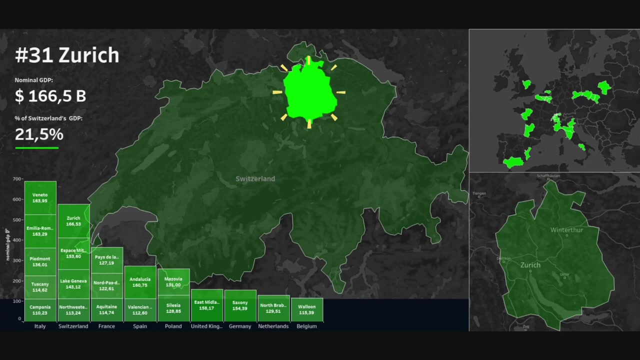 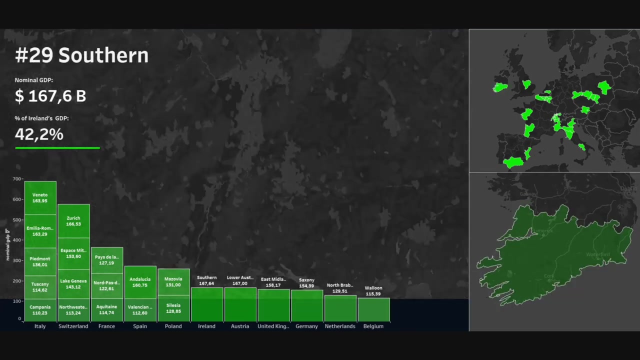 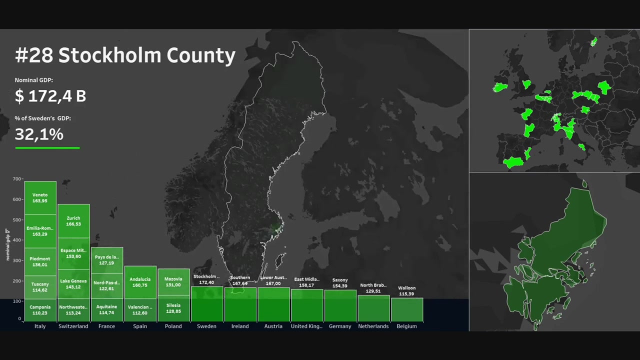 orders were set out. The canton of Zurich is a leader within Switzerland and ranks among the leading European regions in terms of GDP, although its area is one of the smallest in our ranking. It's hard to imagine, but almost a third of Sweden's total GDP is located within a small 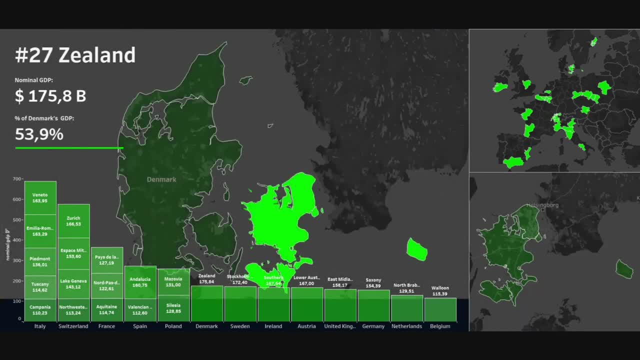 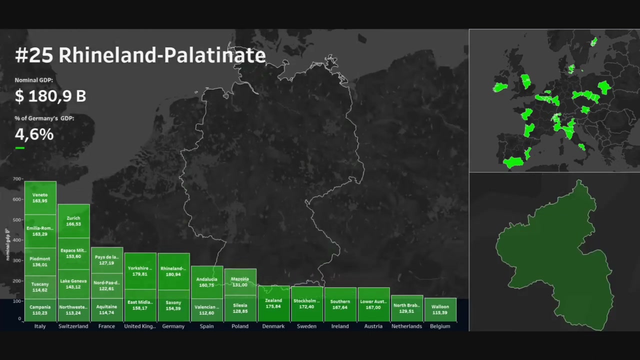 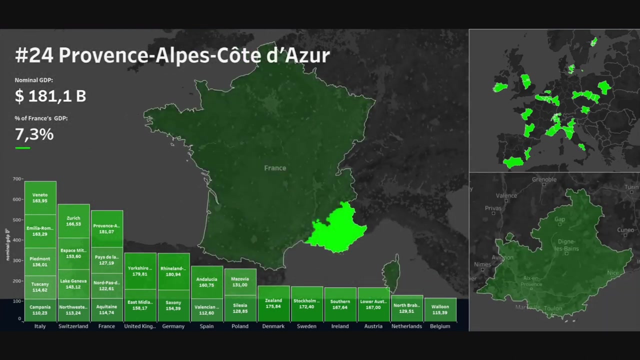 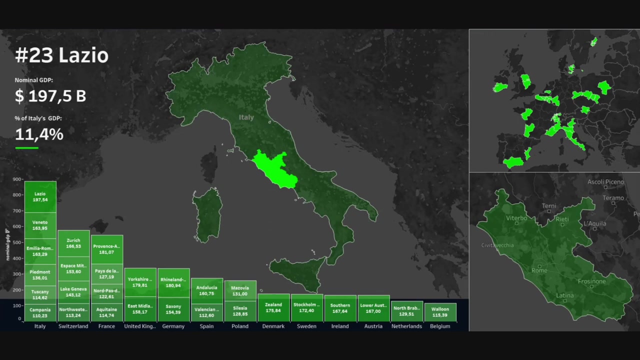 capital district Zealand, including Copenhagen, shows an even greater contrast. This region in general produces more than half of Denmark's total GDP. Lazio is in 23rd place with a GDP of almost $200 billion. Italy is one of only two countries in our ranking where the capital region is not a. 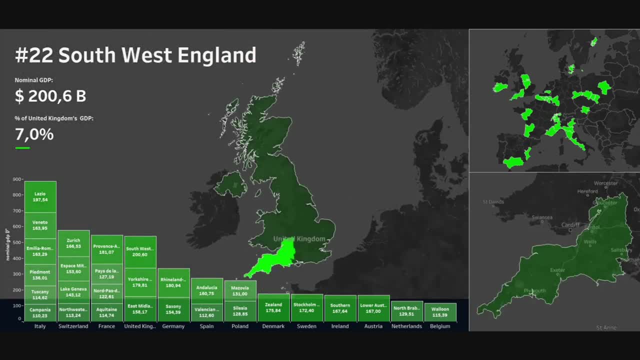 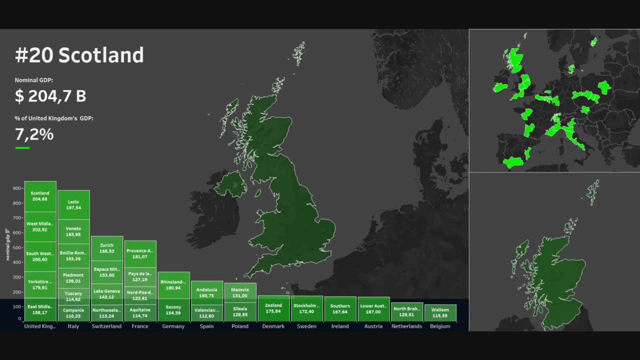 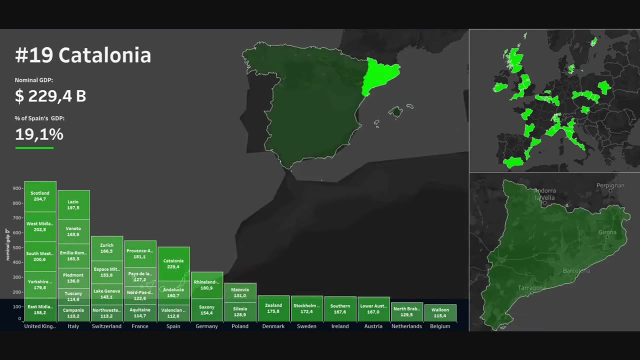 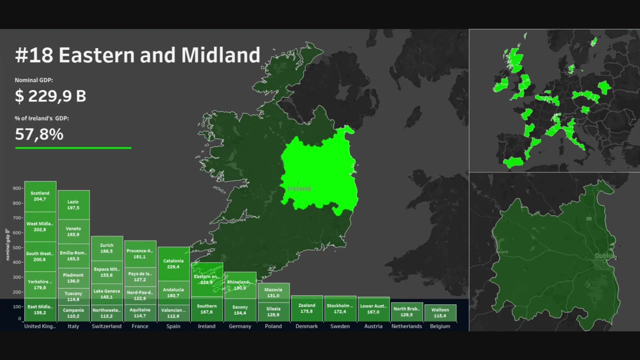 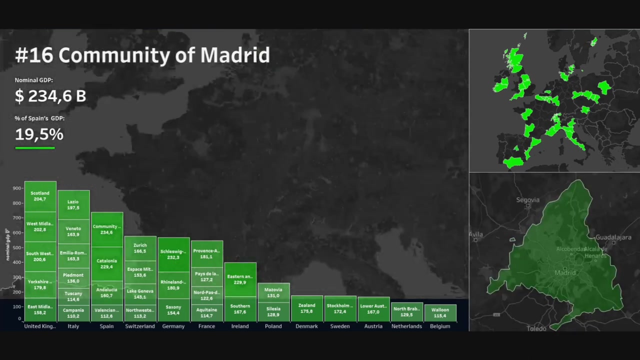 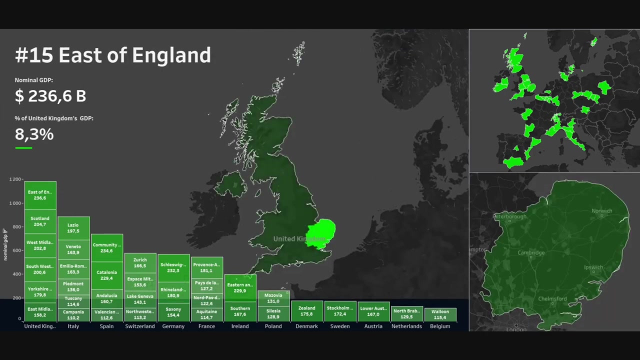 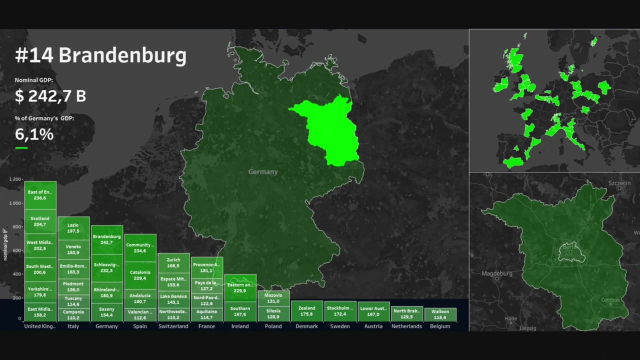 leader within the country. The two countries in our ranking are Germany, Germany, Germany, Germany Germany and Germany. Brandenburg, including Berlin, produces only 6% of Germany's GDP. Imagine how powerful and distributed this country's economy is. 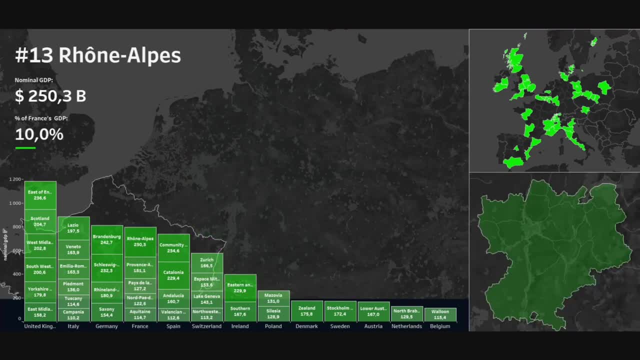 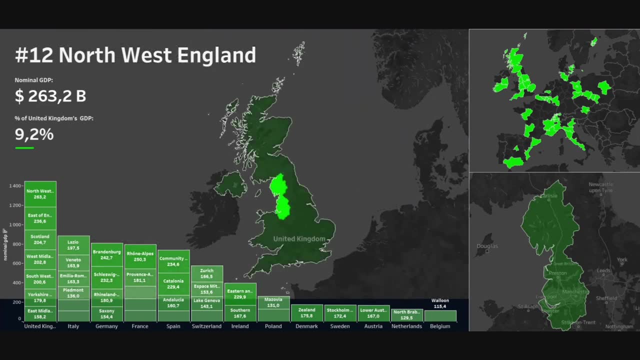 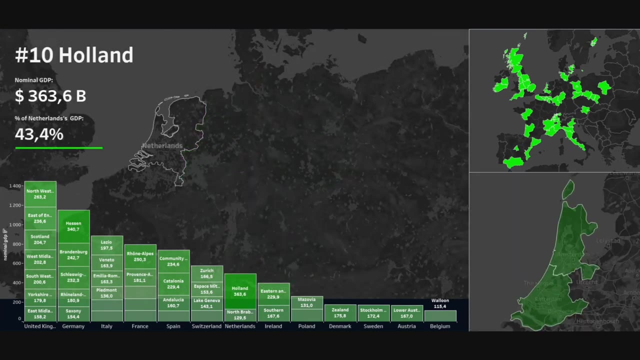 Brandenburg, including Berlin, produces only 6% of Germany's GDP. Imagine how powerful and distributed this country's economy is. The Dutch economy is also one of the biggest in the world. Holland opens the top ten and nearly half of the Dutch economy is located here. 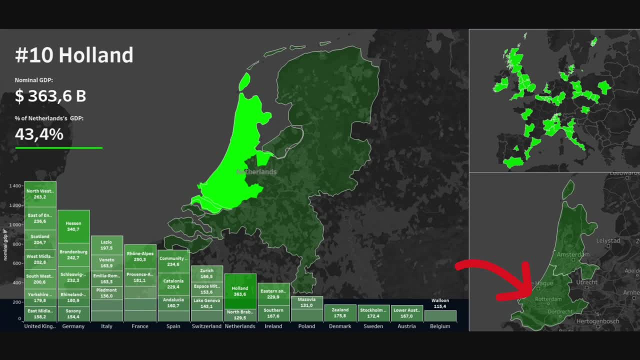 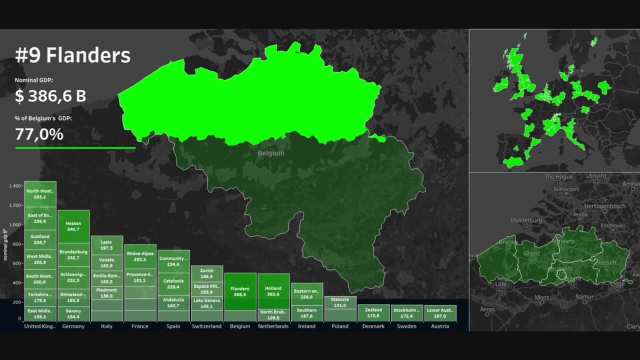 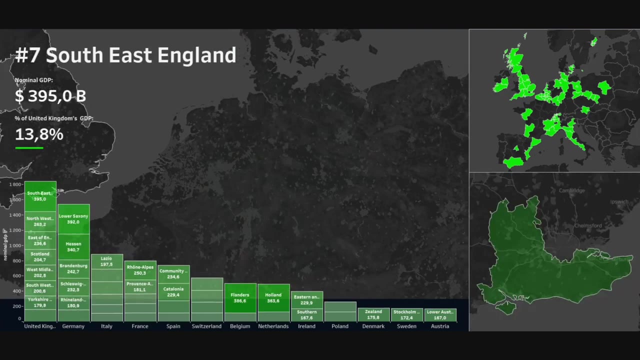 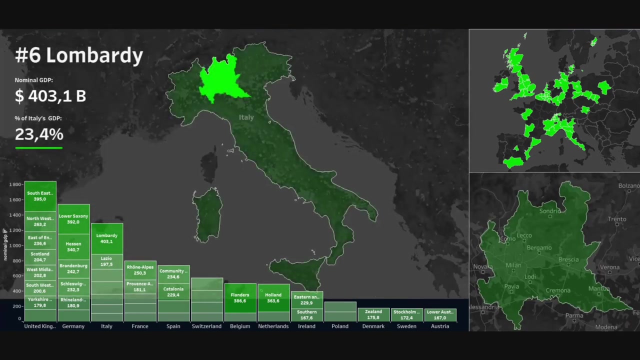 By the way, Rotterdam has long been the largest port in the world in terms of cargo turnover. Flanders, including Brussels, produces an incredible 77% of Belgian GDP. Lombardy is the most powerful region of Italy. Milan is not only the center of 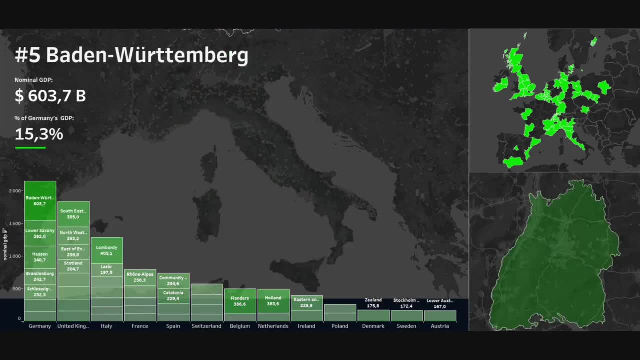 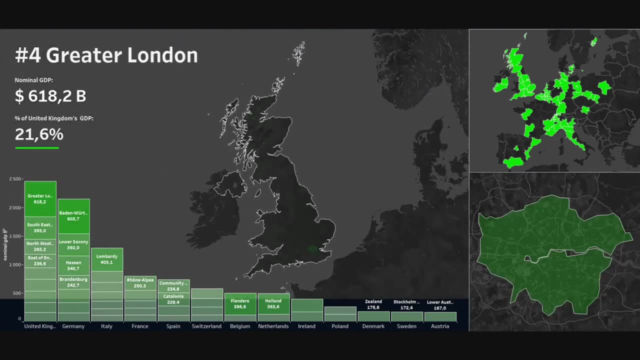 the region, but also the center of world fashion. The top five is opened by one of the three German giants: Baden-Württemberg, centered in Stuttgart. Greater London is on the fourth place: more than $600 billion in GDP, which is higher than countries such as Israel, Belgium and Thailand. 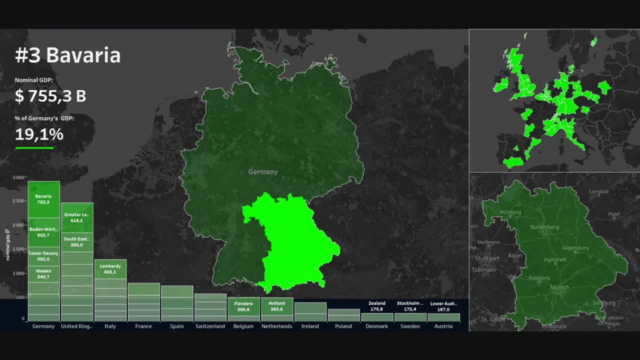 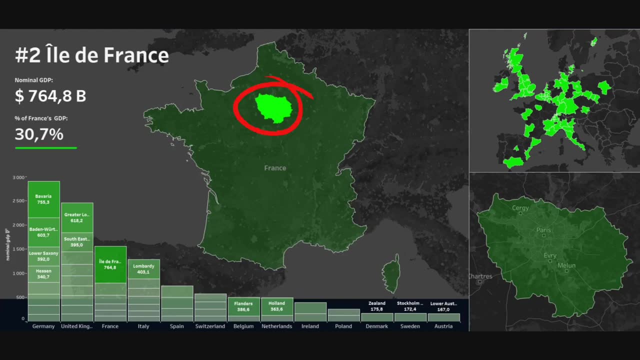 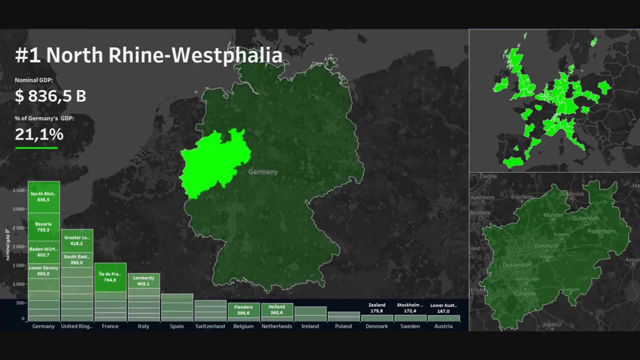 Bavaria is in third place with the GDP commensurate with Poland. Ildi France is in second place. Almost a third of France's total GDP is concentrated in a small metropolitan area. It's incredible. North Rhine-Westphalia ranks first, with an annual GDP of $836 billion. 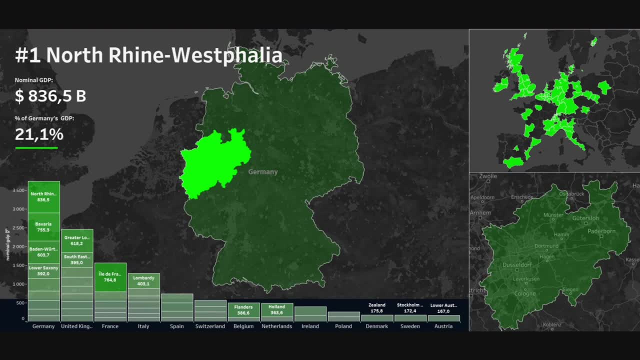 This region is more like a continuous agglomeration of economically developed cities. It is home to about 18 million people, making it the most populous region in Europe. That's all for today. I hope the video was useful for you and you improved your knowledge.